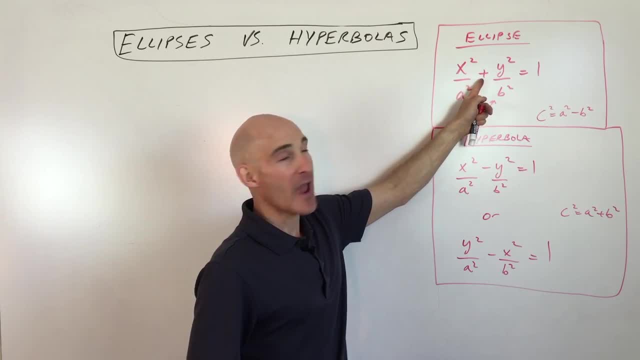 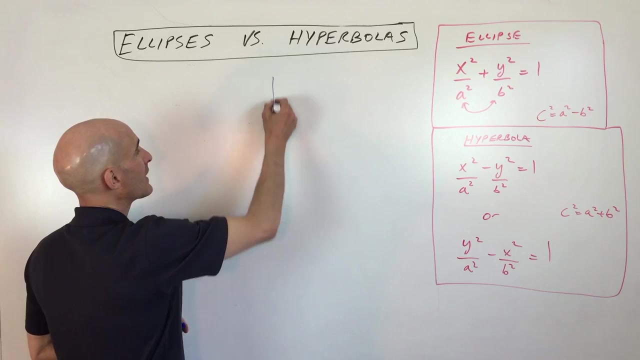 Ellipses. what you'll notice is that you're adding With hyperbolas. you'll notice that you're subtracting Both of the equations. they equal one and they both have these denominators of a squared and b squared. So let's look at an ellipse and we'll just kind of look. 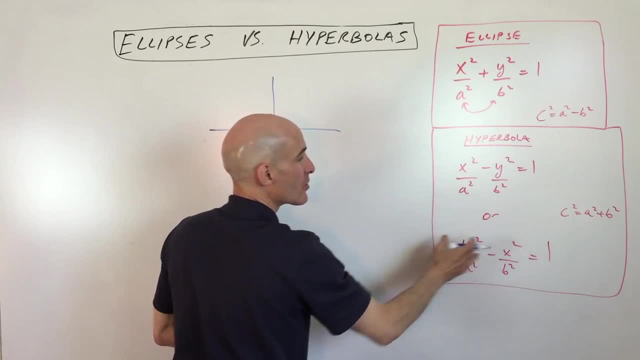 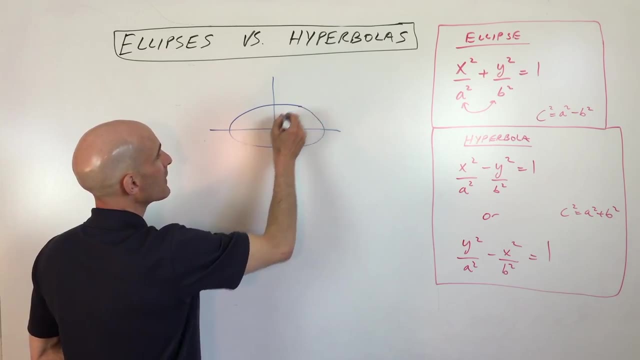 at the anatomy of an ellipse. These ones that I've drawn here are centered about the origin, So that means the center is right at the origin. So if I draw an ellipse like this, here's the center, The distance from the center to the vertices. okay, I'll just write vertex. 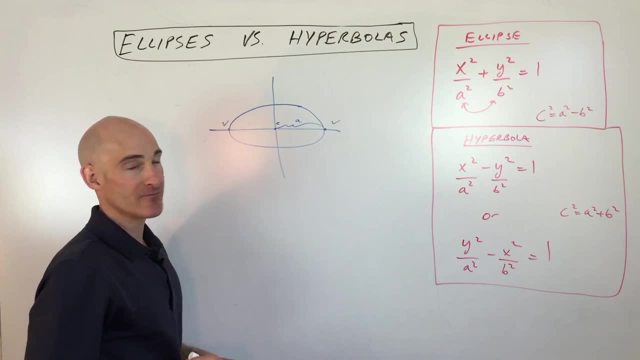 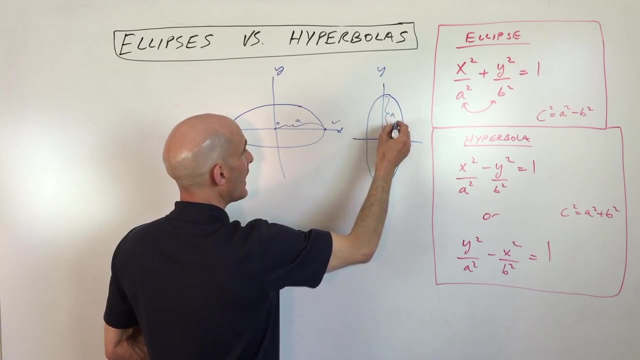 here that distance is called a. Now, it's possible that the ellipse could be longer in the y direction, okay, in the vertical direction, And in that case this is going to be a okay, and this distance to the minor vertices, or the co-vertices, that distance. 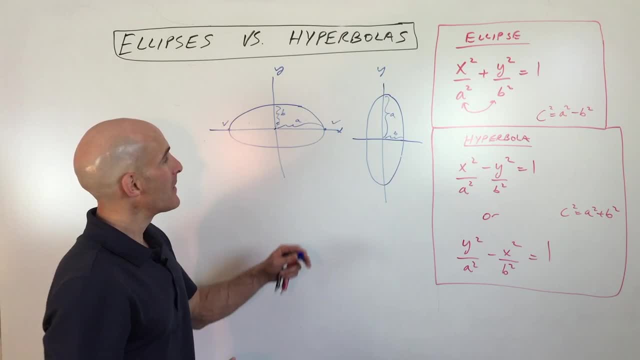 is called a, And in that case this is going to be a. okay, and this distance to the minor vertices, or the co-vertices, that distance is called b. So are you with me so far? I'll give you some examples of the equation. So say, for example, this one could be x squared. 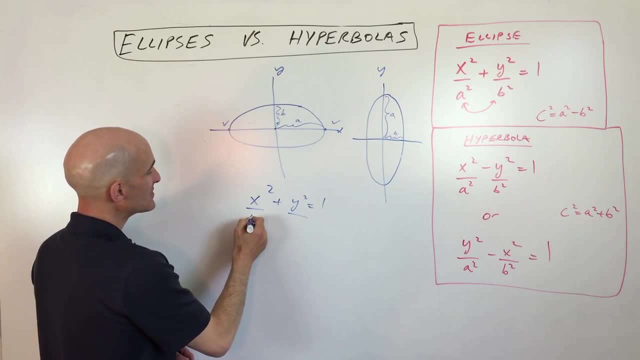 plus y squared equals one, And this is going to be maybe, let's say 25 and let's just say 16.. So what that means is that I'm going five to the right and five to the left. So the number underneath the x tells you you're going in the x direction. So it's easy to. 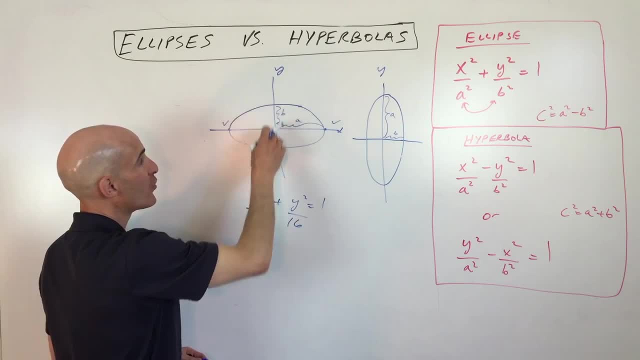 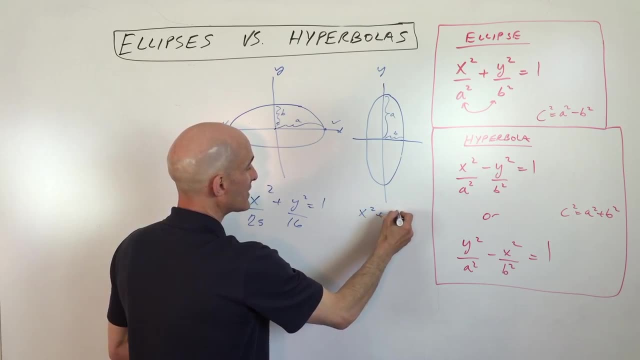 remember right- Whereas the number underneath the y that tells you you're going to be going in the y direction, Plus or minus four. This one here might look something like this: X squared plus y squared equals one, But the y squared, let's say maybe, is 100, whereas the x squared maybe. 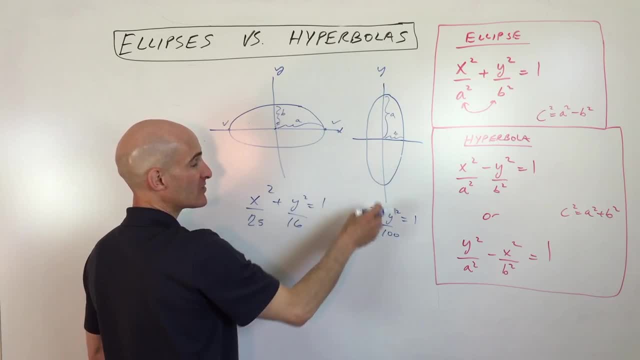 is only nine. So this tells you you're going up 10 and down 10 in the y direction And you're only going three left or right in the x direction. So in this case the larger number is the a squared and the smaller number is the b squared. So this is the larger one. 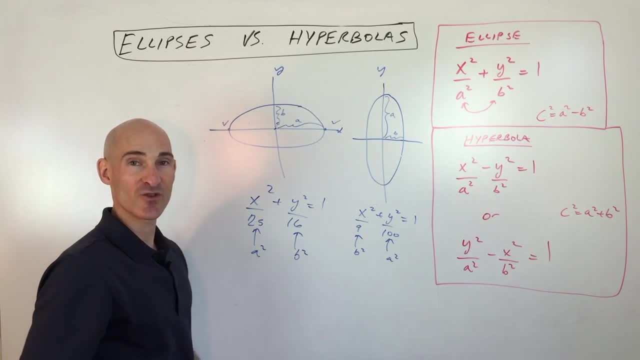 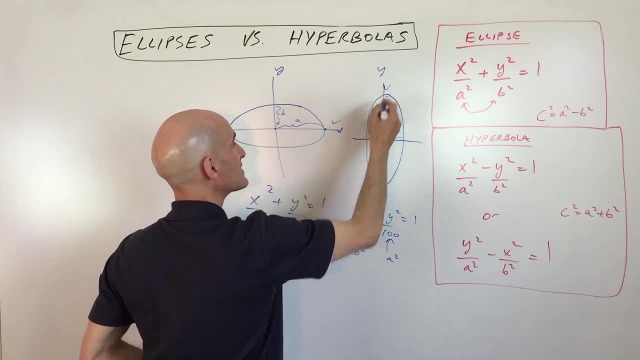 This is going to be the a squared. This is the smaller one. This is the b squared. Are you with me so far? So that's the idea. So the distance from the center to the vertex, center to the vertex, that distance is a center to the co-vertex or minor vertex. That distance is called b. 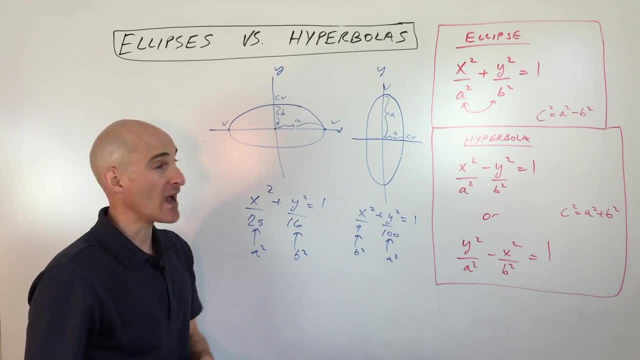 OK, Now the other component are the foci And the foci. that distance is the distance from the center to the focal points, And the focal points are going to be on the major axis, That's the longer axis. That distance is c, And for ellipses we use the formula: 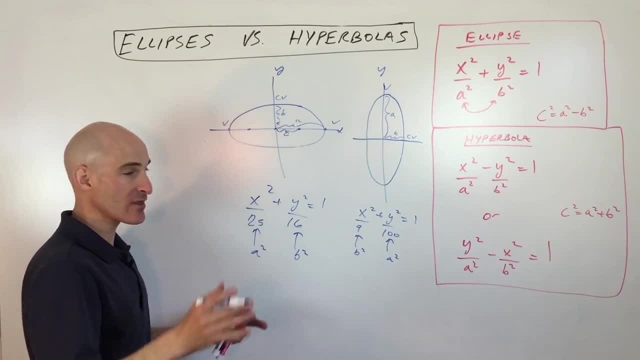 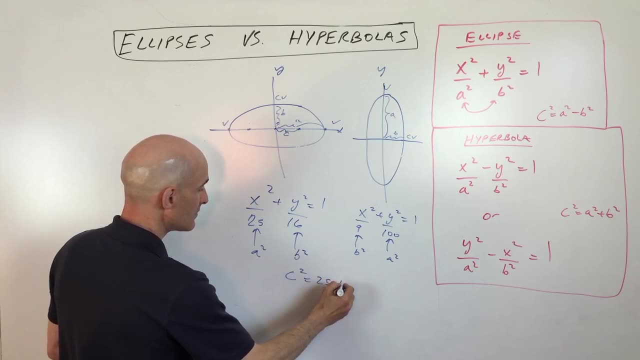 c squared equals one. So a squared minus b squared, Kind of like Pythagorean theorem. but you're subtracting, So for this one it's going to be: c squared equals 25 minus 16, which equals 9.. And if 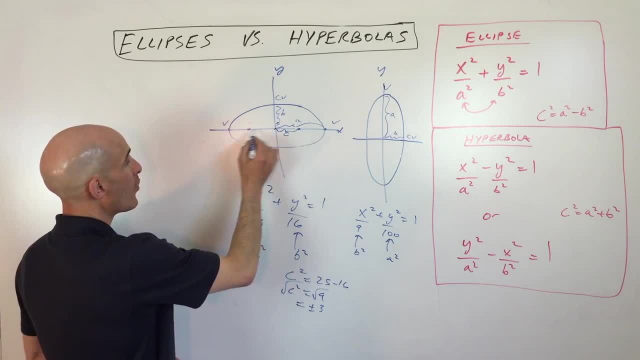 we take the square root of both sides, we get plus or minus 3.. So you want to make sure that the foci f are on the longer axis. So we're going to be going right three and left three, And that's how we find the foci For this one, since. 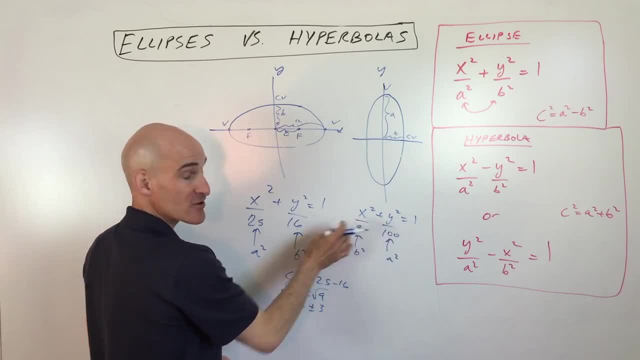 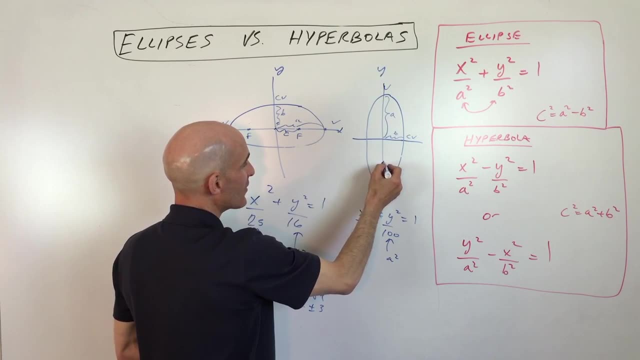 it's orientated vertically Because the number underneath the y squared is larger than the number underneath the x squared. this is our major axis, This is our minor axis. Our foci are going to lie along this axis, like this, And again, what we would do is we would do: c squared equals a squared. 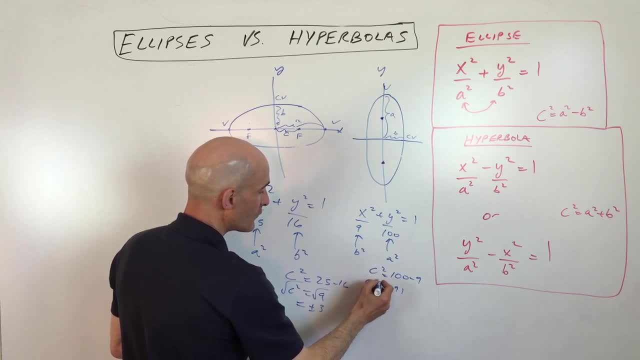 minus b squared, This comes out to 91. And if we take the square root we get plus or minus the square root of 91. So that's going to be. they actually would be a little bit higher, like this, OK, and a little bit lower. So those are the foci. 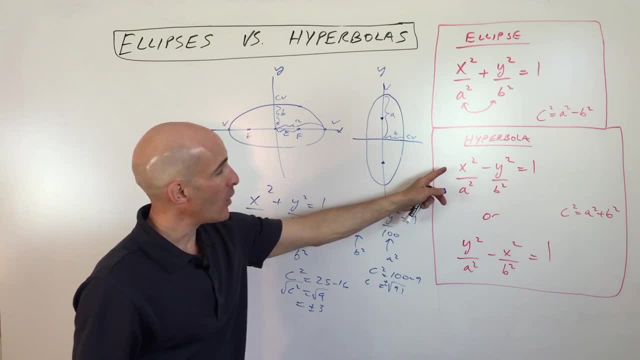 OK, Now we're going to switch gears to talk about hyperbolas. Now, hyperbolas, whichever one comes first, that's the positive term That tells us which direction the hyperbola is going to open. If it's x squared, that comes first, it's going. 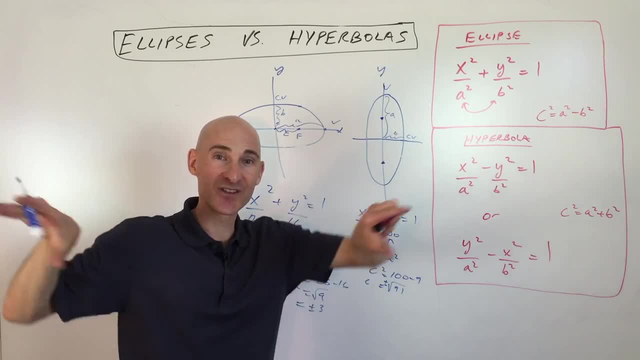 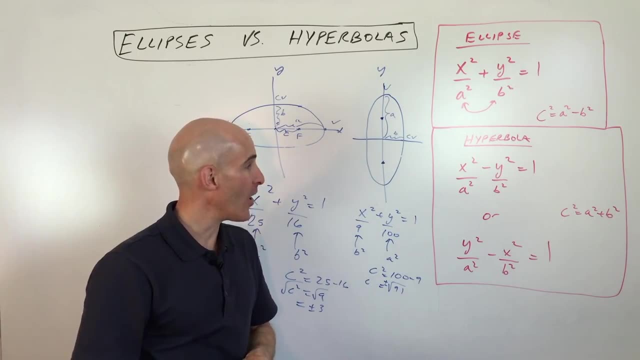 to be opening in the x direction. Like the x axis goes horizontal, it's going to open horizontally If the y squared is first. it's going to be opening in the direction that the y axis is, That's, vertically up and down. So let's look at an example. Let's take this. 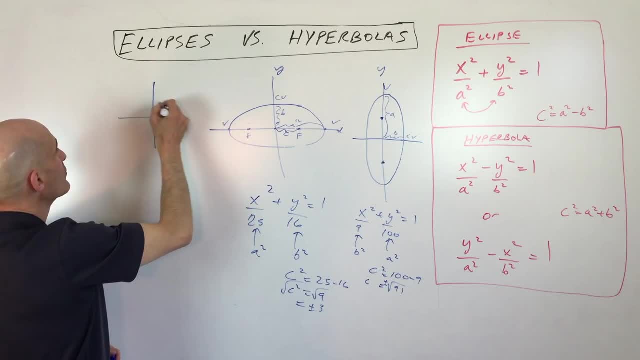 first one over here, Say, we wanted to graph a hyperbola that looks like this and like this. So what we have is x squared minus y squared equals 1, OK. just like ellipses, they equal 1.. But this one that we're going to say maybe, is 4 and 1.. OK, So what the a squared is for. 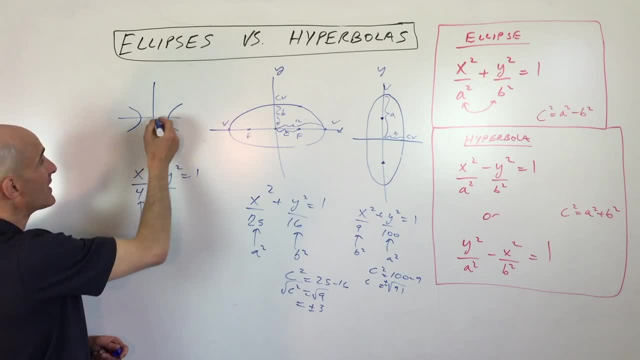 this problem is going to be 4.. So that means that a equals plus or minus 2.. So we're going to be going right 2 and left 2.. That distance is our a value, That's the distance from the center to the vertices. 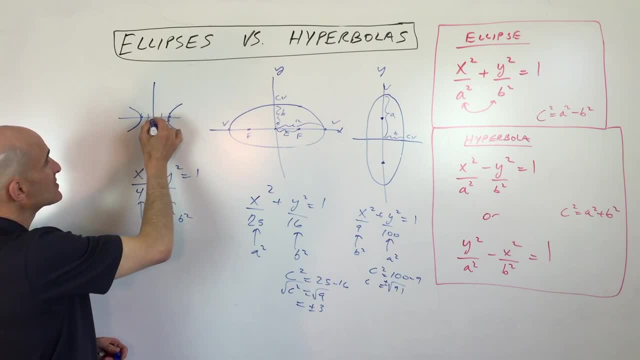 Now, if we want to, this will be the b squared here- And if we want to find the distance to the foci, the foci are going to be along that major axis, OK, the same axis that the vertices are on. We're going to use the formula: c squared equals a squared plus b squared, just like. 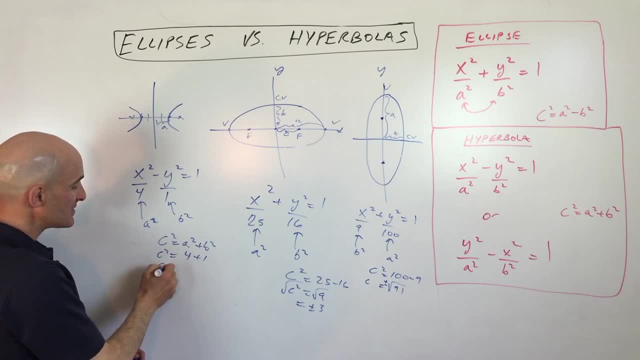 Pythagorean theorem And that's going to be: 4 plus 1, c squared equals 5, c equals plus or minus the square root of 5, which is about, maybe right about over here and over here. OK, So just a little bit further out from the center. 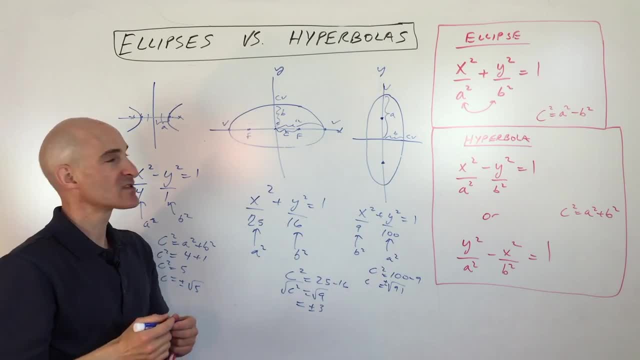 Now some students. they'll kind of make these little notes to themselves. They'll say, hmm, so with ellipses the foci are close to the center. So they'll say, hmm, so with ellipses the foci are close to the center, they're on the inside. With hyperbolas, the foci are 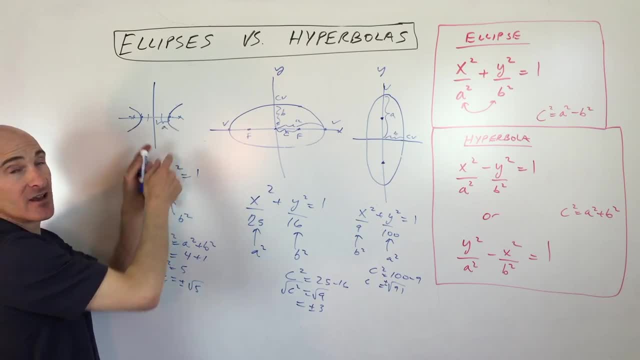 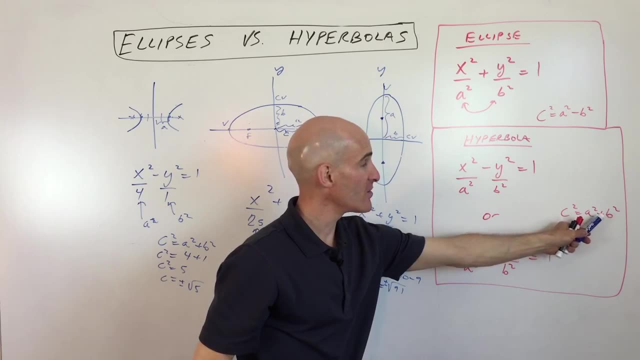 further out from the center, They're going to be on the outside. And the other way the students oftentimes remember these formulas is that hyperbola you're subtracting, but in your focused formula you're adding is the opposite. With ellipses, you're adding: 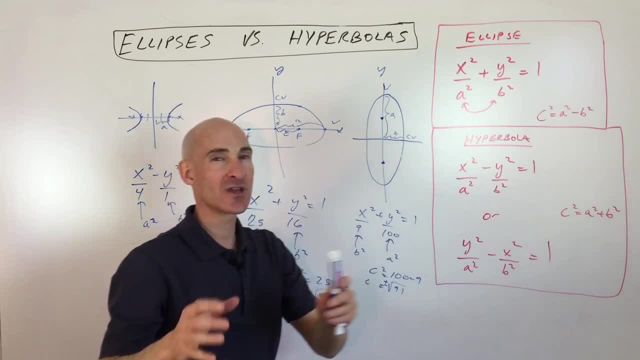 here, but in your focus formula you're subtracting. So I'm just trying to give you some hints or ways of remembering these different formulas. Let's look at one more example with hyperbolas. This is a simple formula. again, This one you'll see for just about any particular single capsule. 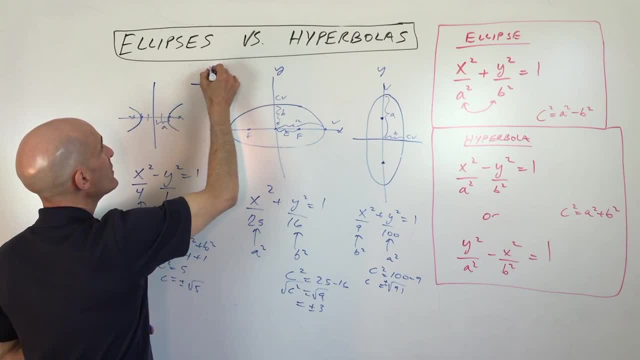 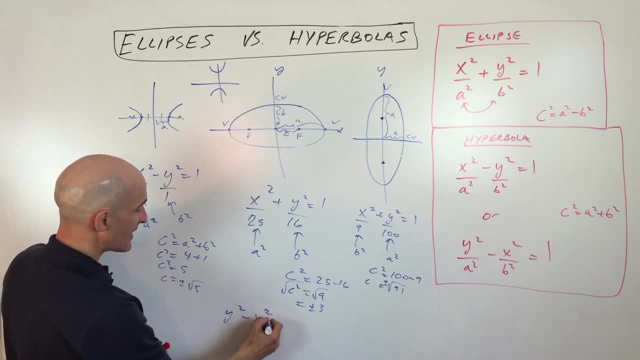 Let's look at the case where we're now adding our object, which is flat Bella, and when you're, let's see if we can fit it in right here. if it's opening like this up and down, that means that it's a y squared variety. so I'll write it down here: y squared minus x squared equals.